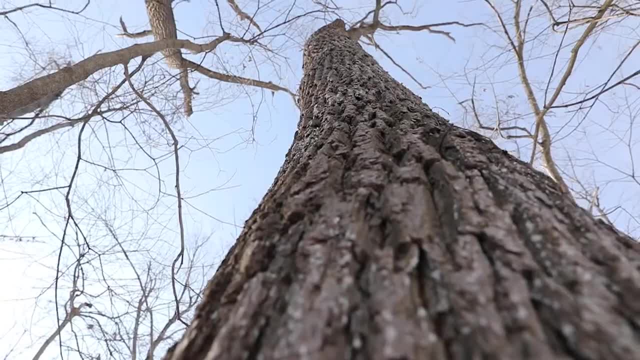 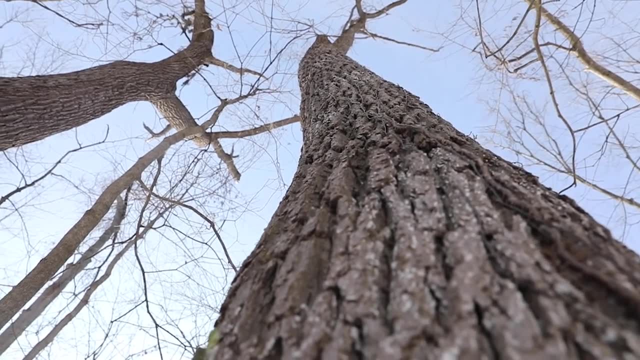 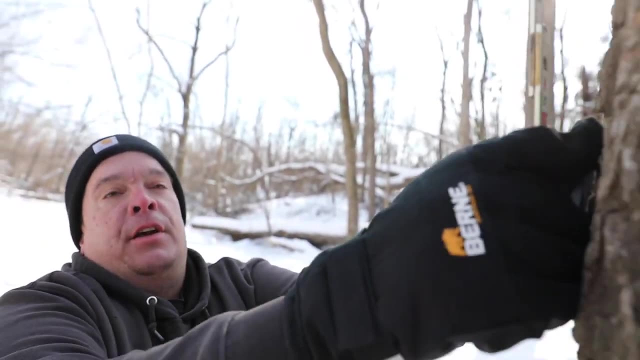 merchantable volume of logs within the tree from two measurements: diameter and merchantable height. Soon we'll see Ben recording these measurements for a black walnut. Once he's obtained diameter and height, he'll use a tree scale volume table to further adjust his estimate for accuracy. Why use 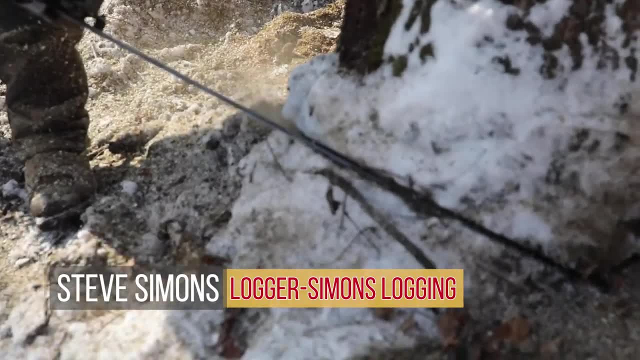 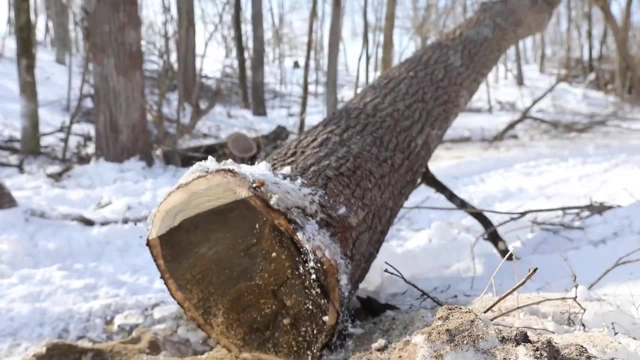 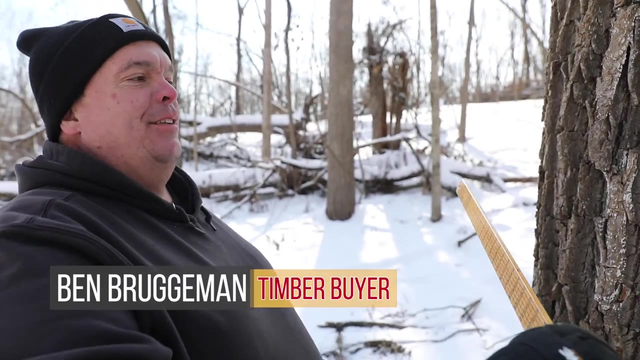 a volume table. Why not just calculate the volume of a cylinder? Well, trees and the logs they produce are not perfect cylinders, so volume tables help increase accuracy by accounting for factors such as log taper and bark thickness. We're going to measure the log with a from the left to the right, using these measurements to get the correct volume and height of a tree table. 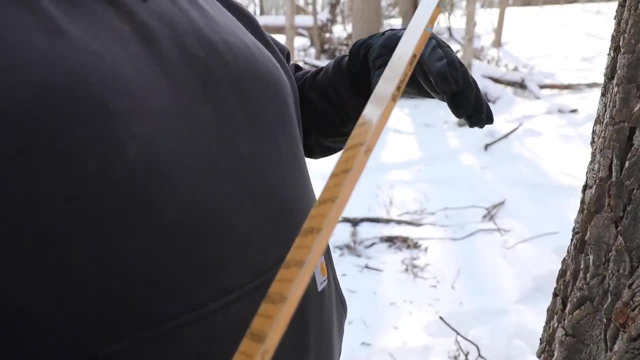 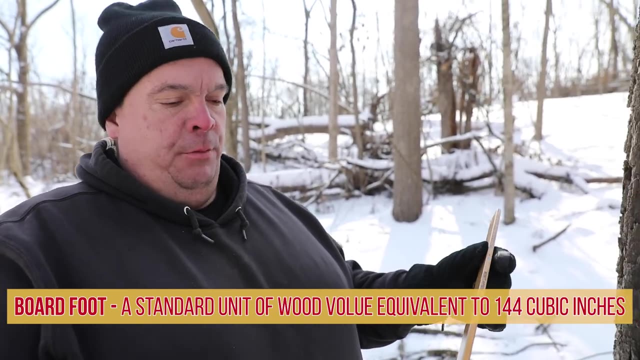 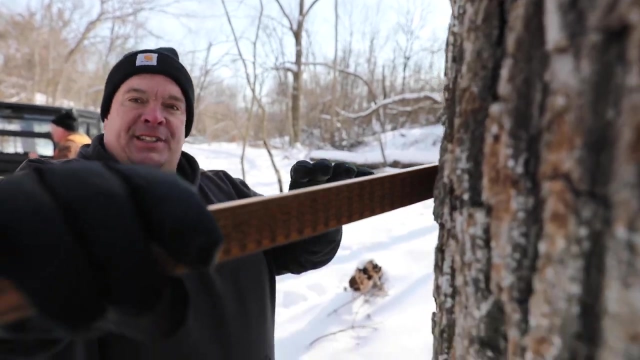 a tree stick and uh to figure out the board feet of the tree when it's standing. it's all, no matter who does it, it's all just. they're merely an estimate, but you keep the stick more or less the arm length away, at four and a half feet, or you know breast height, depending on how you. 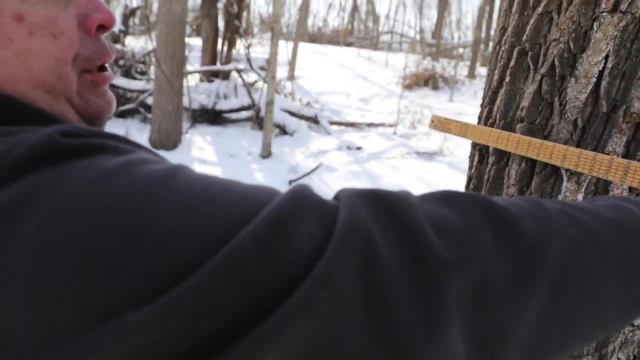 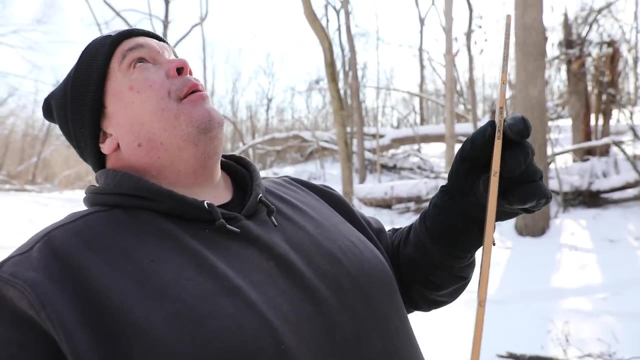 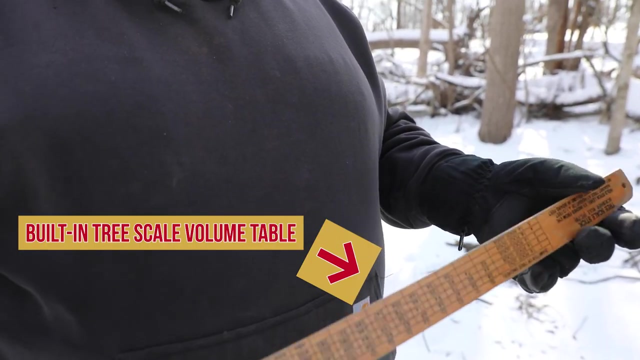 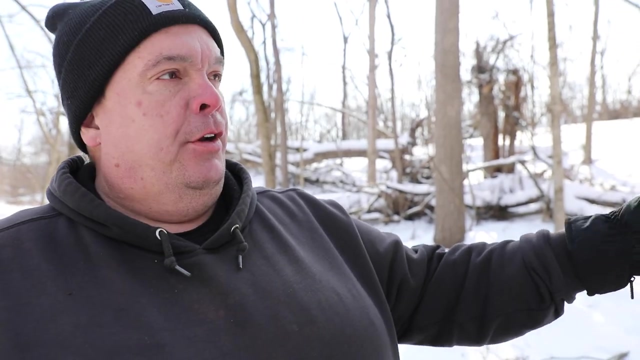 tally are. so if you this tree, uh, you could say it's a 19 inch tree, that's diameter up, you know, outside bark, and uh, if you look up, it's a, probably a log and a half, uh, 24 feet. it's not quite long enough for two. so this tree would be 200, probably 200 board feet is a, you know. 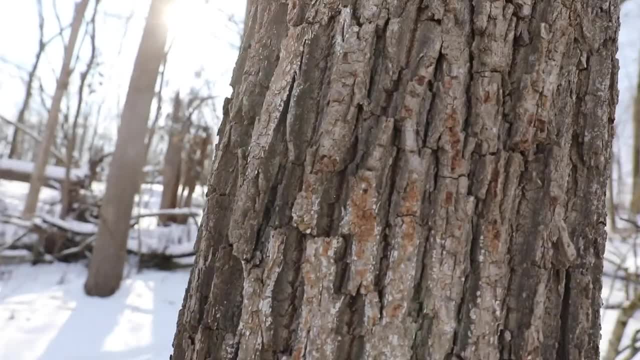 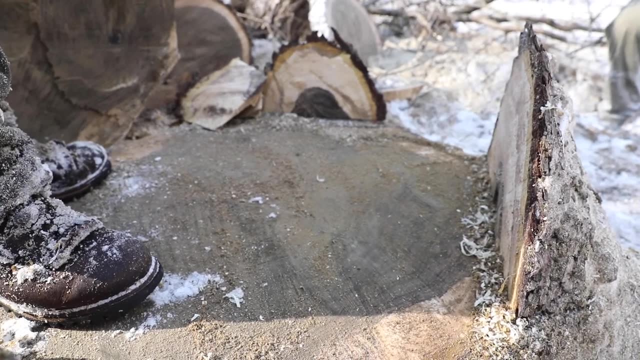 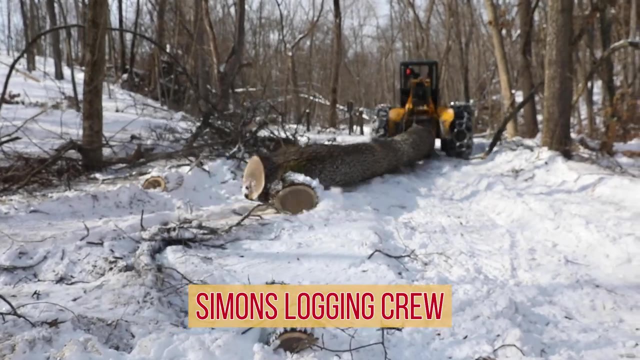 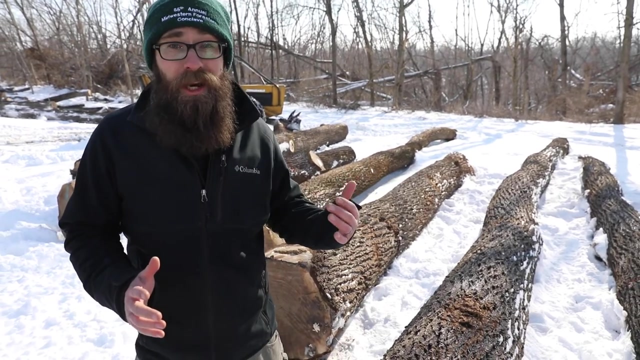 estimated board footage for this tree. once scaled by a professional forester, loggers harvest the trees and transfer them to the log landing. the process of carefully removing logs from the wood is also called skidding. once at the landing, logs will undergo further scaling and grading from log buyers. we're up here now at the log landing, so they've drug or skidded all these. 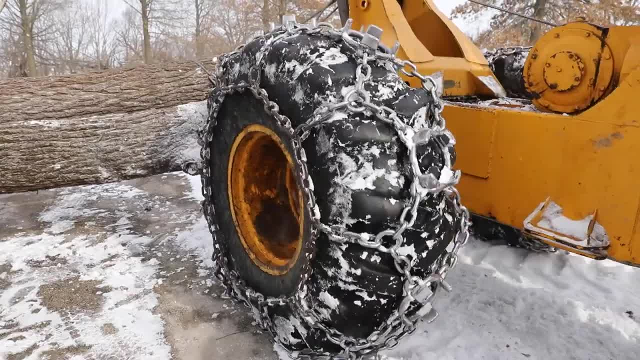 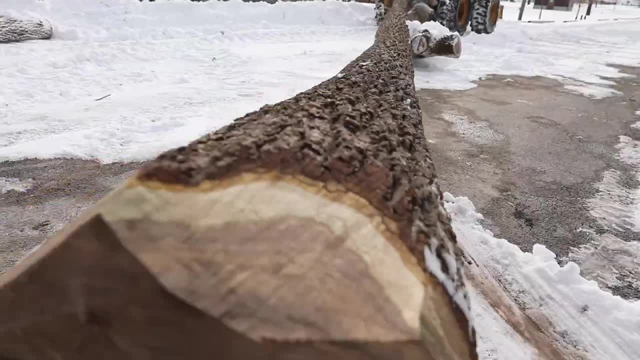 logs out of the woods and placed them here side by side. it's an impressive site with all these high quality black walnuts here, but these logs are now just waiting for timber buyers to come and examine them, scale them and see if it's the quality and amount that they want to purchase. 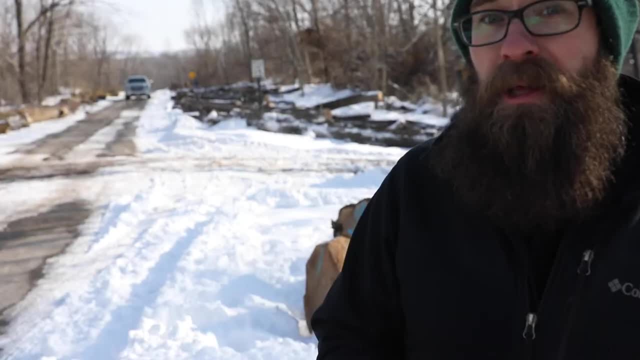 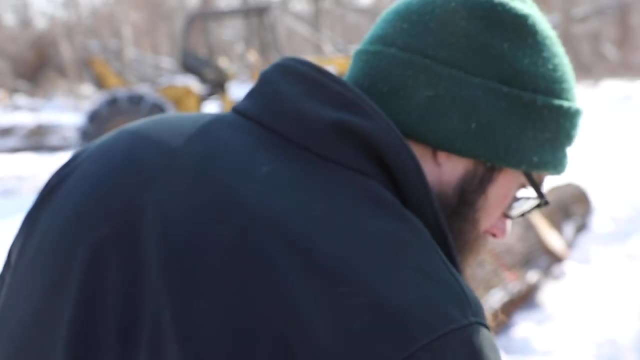 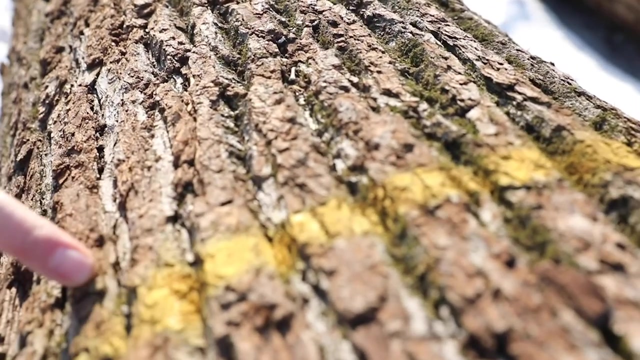 in the background. here we can actually see a buyer scaling the logs right now to see if it's the quality and that they're looking for. a lot can happen to a log during harvest, so once on, the landing logs are scaled again for volume. next, ben explains why. 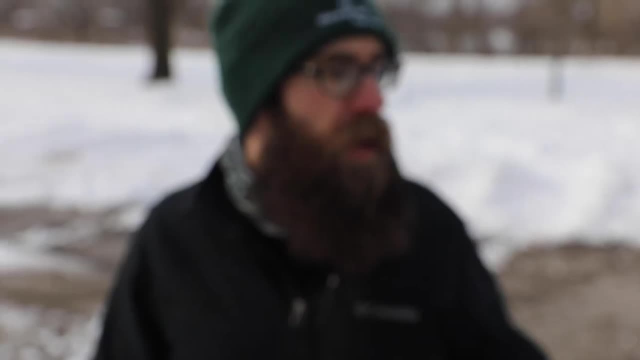 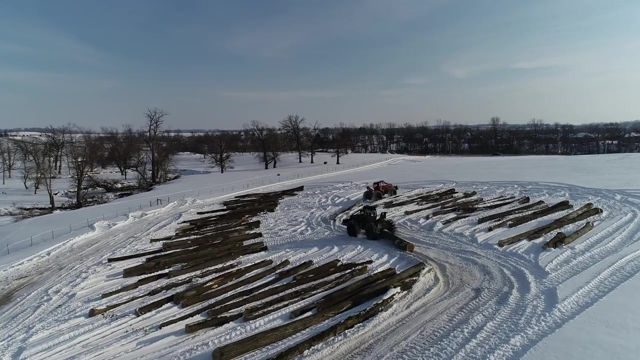 a second scaling at the landing is necessary. well, ben, we've skidded this out. we scaled it in the woods. um, now we're going to scale it again and i'm just curious: what are some of the differences you see from in the fields up in the landing here? um, so the truth is we're going to scale the logs. 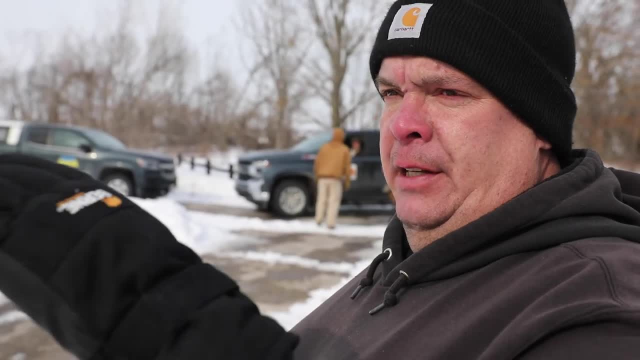 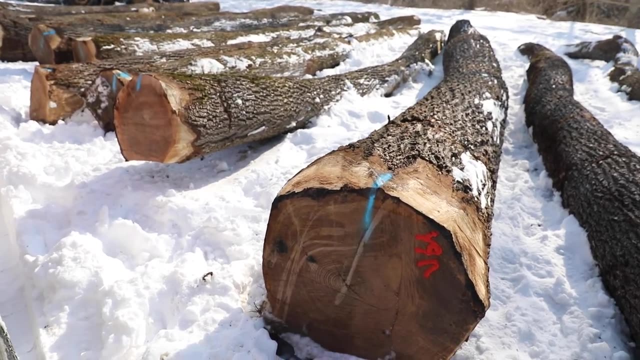 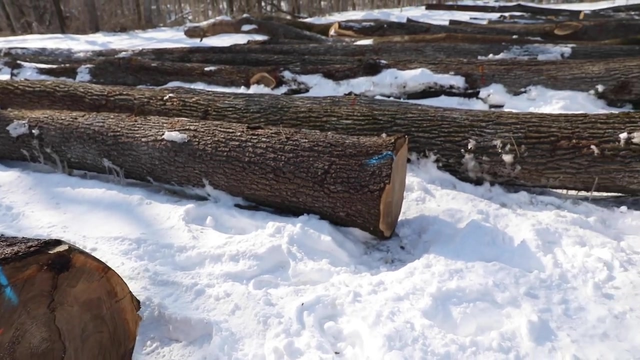 in the woods it's hard to calibrate the height of the tree versus the you know standing there, and a lot of times when you utilize the tree to the maximum, you bring out logs that you may not have figured, because sometimes when the tree falls, the tree might snap or break those. so you kind of 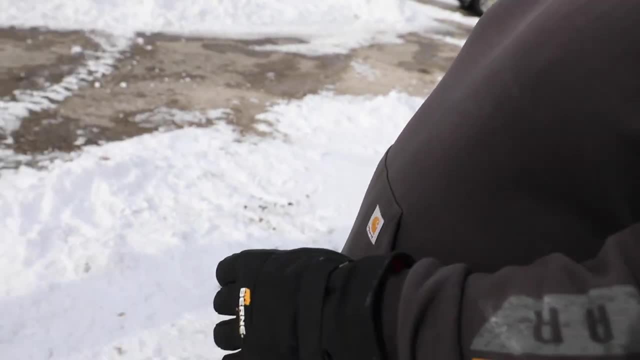 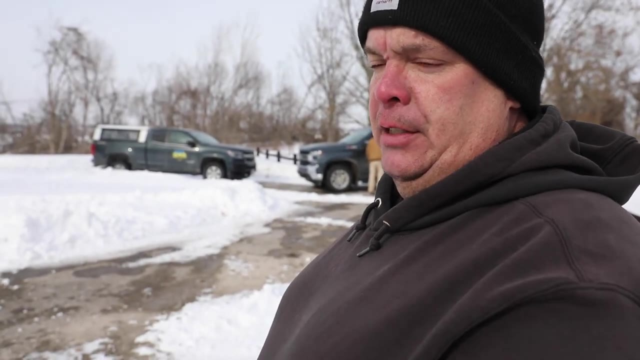 conservatively say: you know, like this tree that we're going to look at here, we called it 24 feet in the woods, not knowing that if those smaller logs up top would break. well, now that we get it to the landing and on a on a grade yield, salvage that we're doing. the more we bring out, the more the landowner is going to receive, and usually i would say maybe 20 percent of the volume that you see in the woods you can gain at times, depending on how the tree was scaled by the, either the forester or you know whomever, because uh. 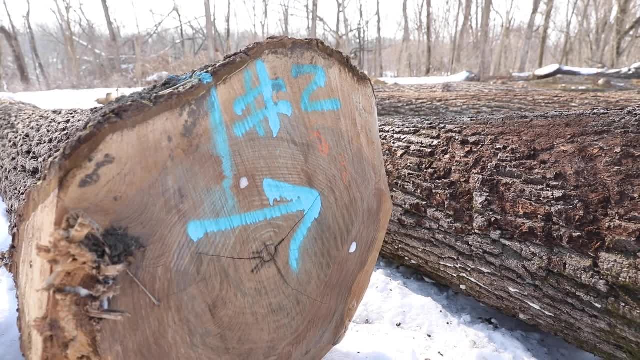 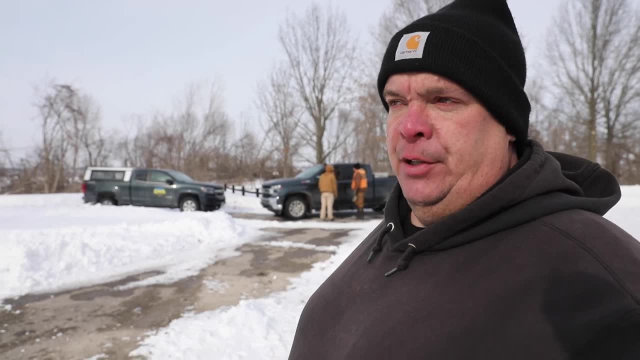 they may claim that they can get all that out, where some people, if it breaks, they can't. so uh, it's always better to err on the side of caution, especially this time of year, when it's cold, the trees are, they tend to break easier. once volume is determined, logs are then graded. 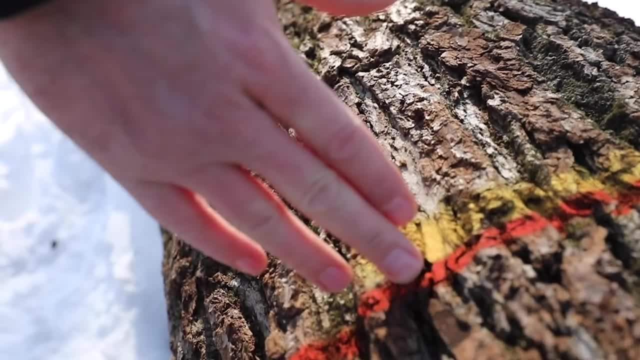 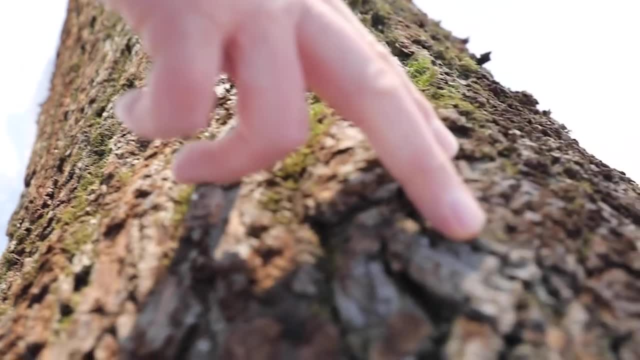 grading entails assessing logs for overall quality and end use and deducting volume associated with any defects. well ben, we've got the logs skidded up here to the landing and a lot of folks are kind of curious what happens between this point in the middle, like: what are the next? 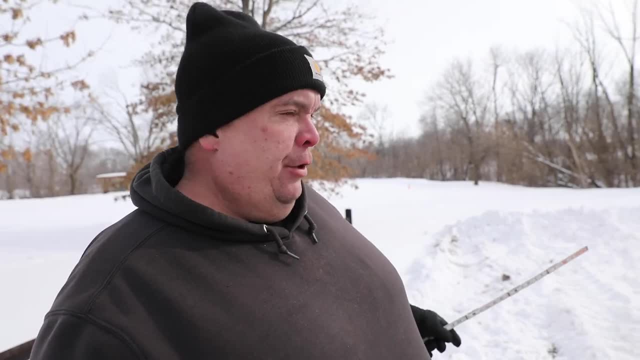 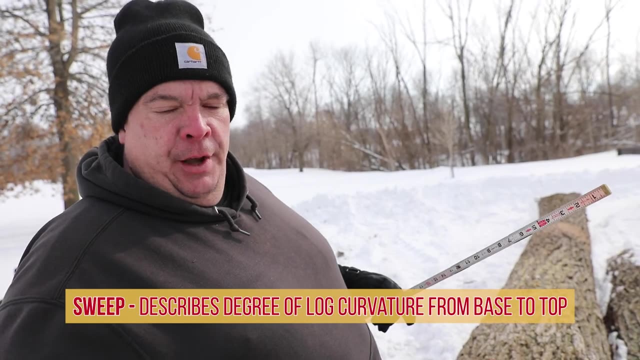 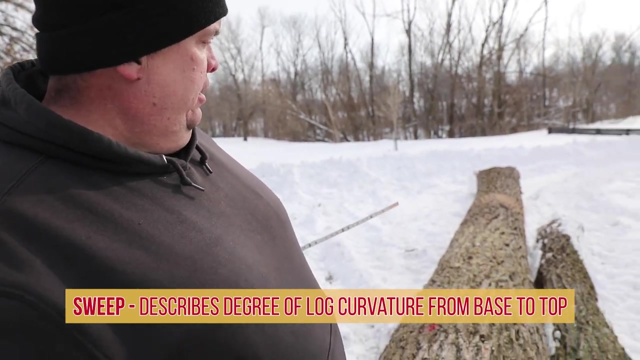 steps here. the first step is you kind of look at the, the trees as they were brung out. you know, in the woods we looked at a tree and i identified sweep and you know other defects. so now that they're here, the, you can physically see them easier because you can get close and you can 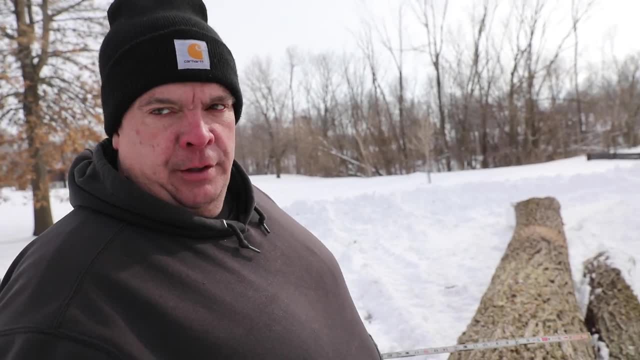 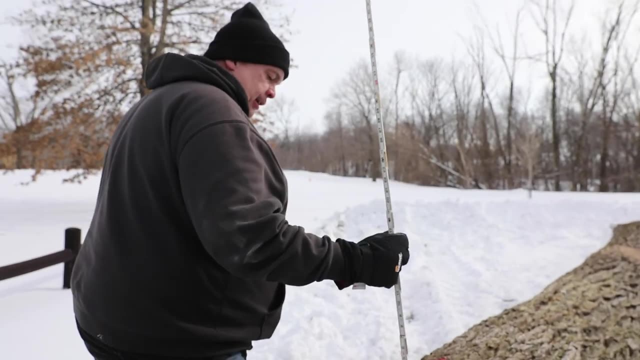 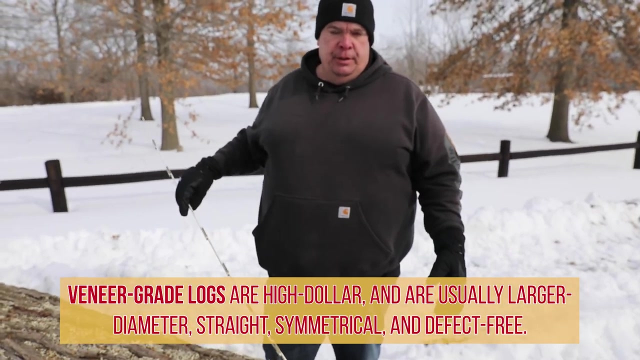 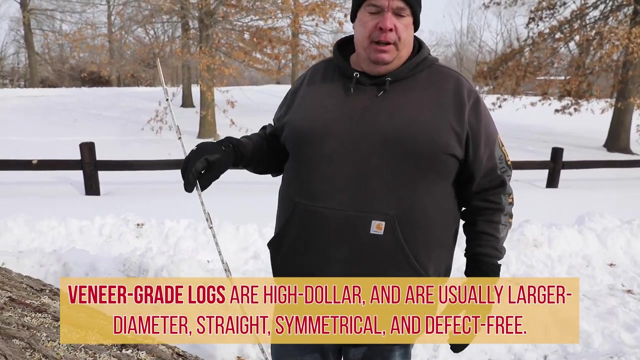 measure them and you get a more accurate reading of the log, because it's now kind of closer to the finished product. um, so what we do is we- uh, you know, mark the, try to mark the log for straightness and quality. veneer is sold domestically and higher end logs, like we're looking at, go overseas, and so the 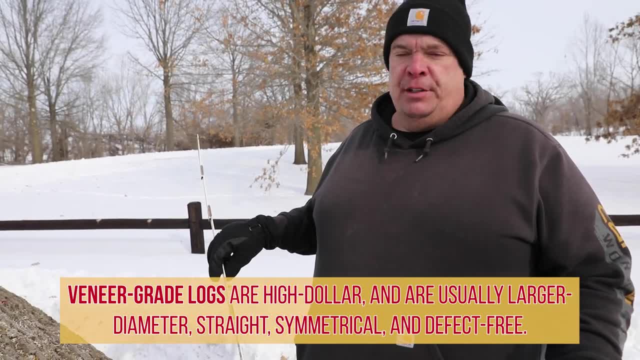 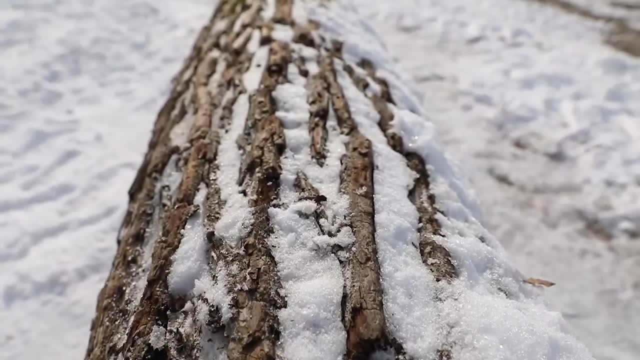 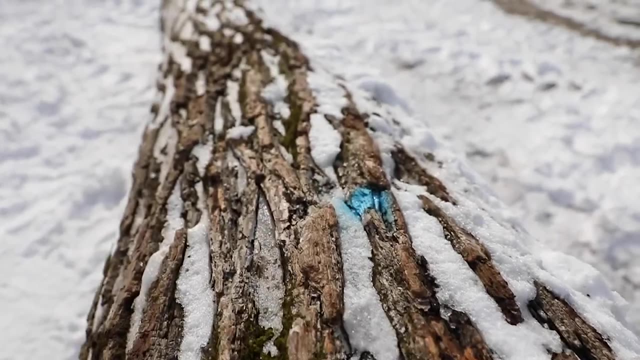 longest log that can be sawed, whether it's domestic or overseas, is typically 13 foot eight. so therefore anything longer than that needs to be four feet longer, so you can make it into a nine or an eight or, but you know, 13 is the longest. so this tree here that we top down in the woods, 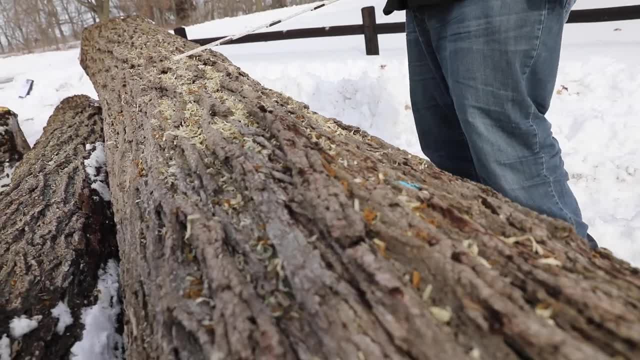 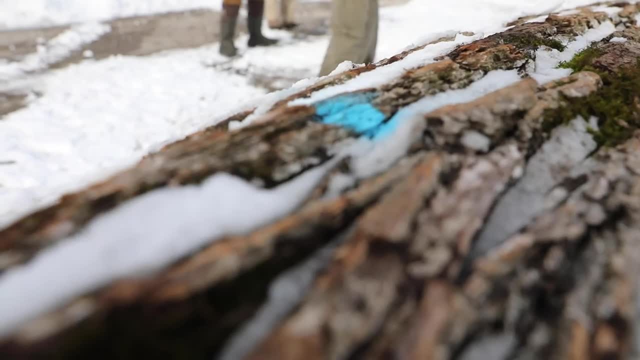 it will make 13 foot to the dot and this is considered a high-end log. so this could either stay here in the united states or, you know, it could go to japan or korea or other countries that buy high-end walnut. it just kind of depends on. 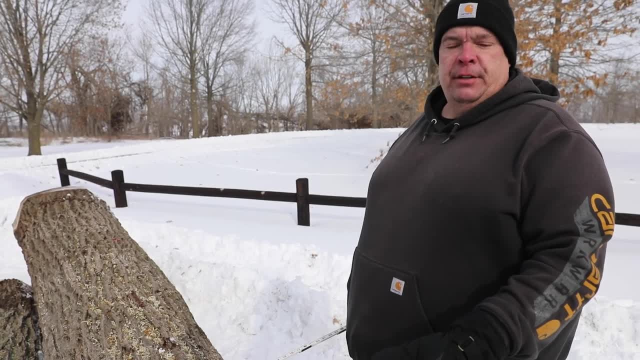 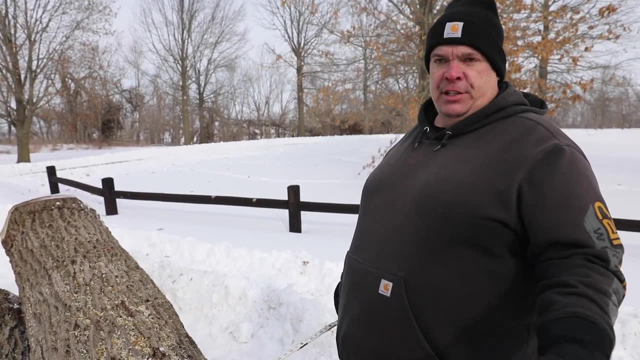 a lot of times the the mill that's domestic- will lay them in their yard and bring a buyer in from overseas and if they pay the price they want, they'll sell it, not even do anything with it. if they don't, then they'll slice it. manufactured here in the united states. 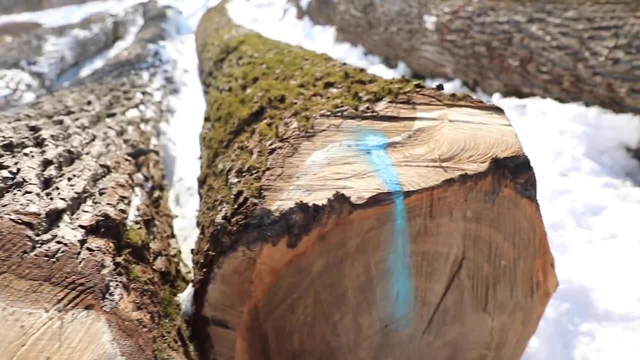 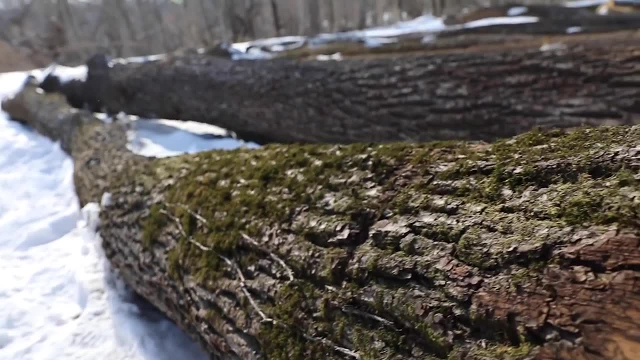 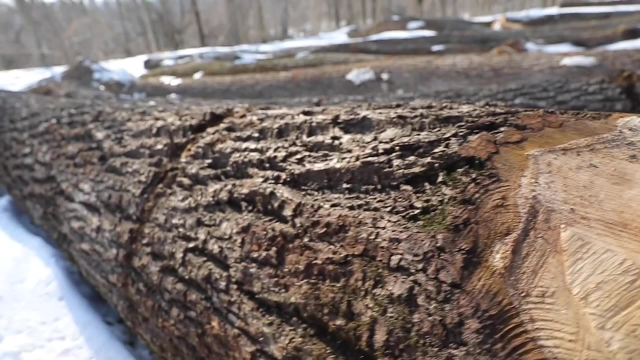 log buyers are highly skilled and can detect the smallest of defects that live beneath the bark. not all defects are bad, however. certain grain patterns, such as those found in branch crotches, are highly coveted by woodworkers and for use in specialty products. but there's a lot of defects. 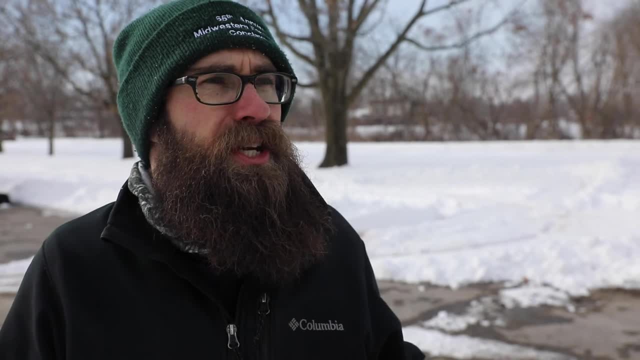 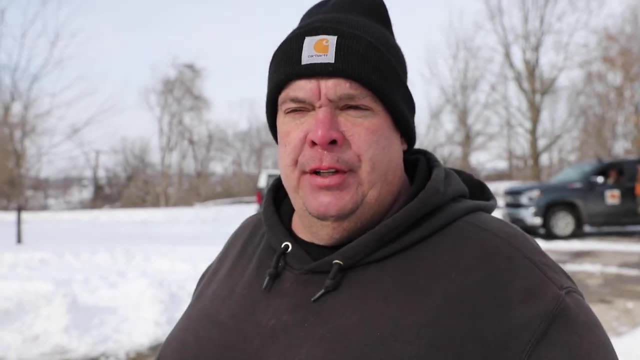 and other conditions that affect the log value. so what were like, say, your top five or six that would really impact the value of that log and describe them? a bird peck is probably the worst and that usually tends to grow in trees that were more open, grown along the edge of the woods. 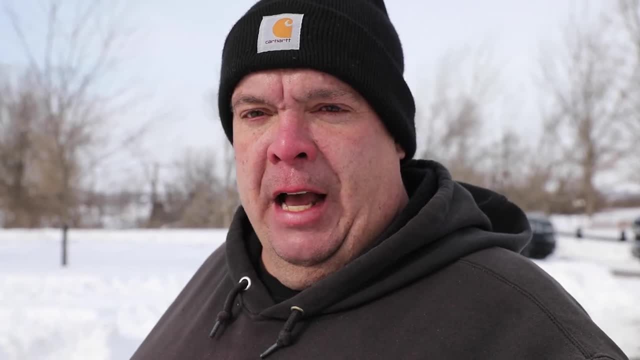 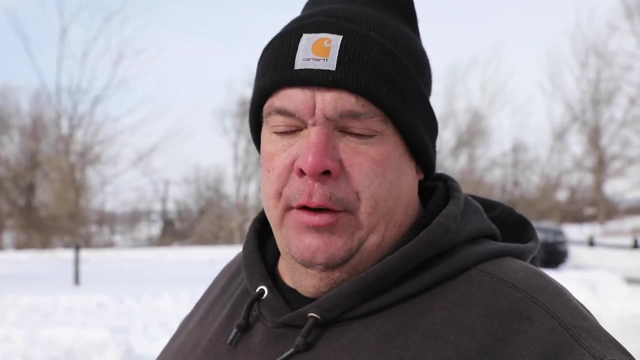 and that bird the peck. it goes into the wood and you can see black dots, which automatically kicks out of any high-grade, you know, veneer In the lumber. it's not quite this bad, but for the most part bird pack is probably the worst. Then you have crook and sweep and that's where the log. 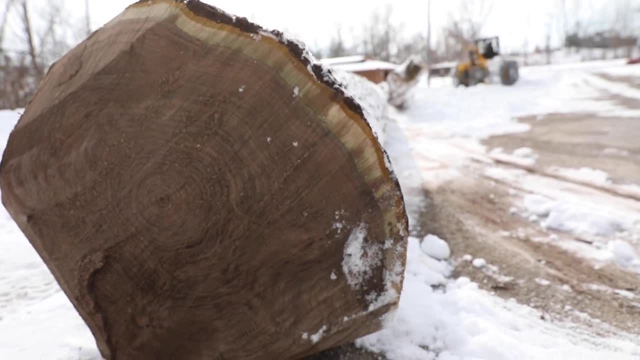 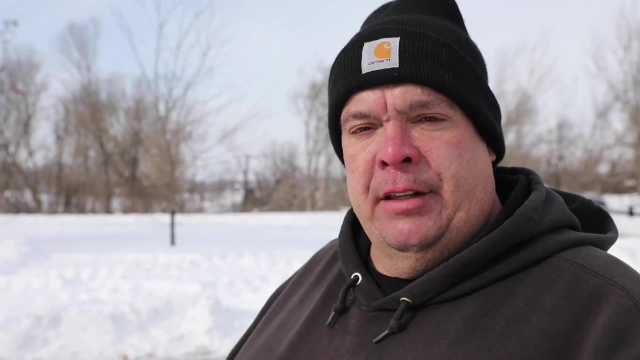 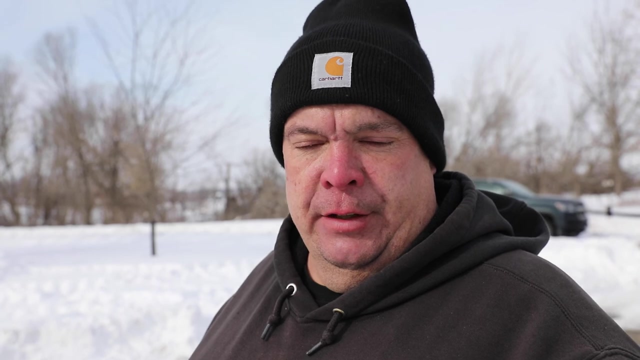 kind of meanders up through the woods to get the sunlight and that affects the wood and the lumber inside of it, because the pith which runs the length of the log, if it's off-centered, that pith will be in all kinds of different boards which affects the yield. So you know, sweep. 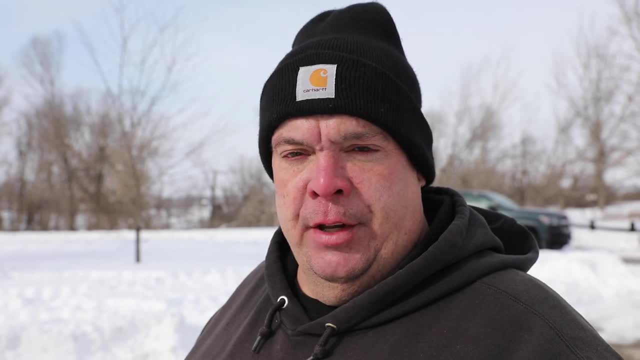 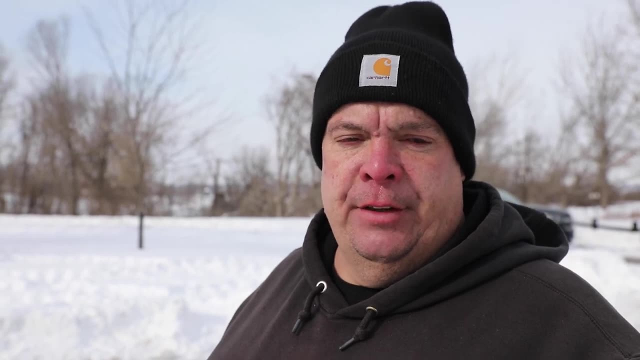 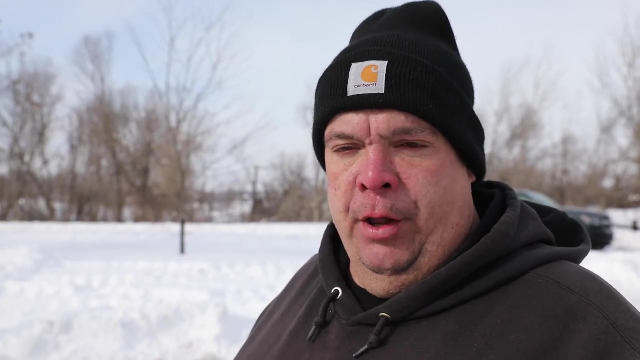 crook. you have pin knots, which you can see sometimes, and it may only be in the bark or in the sapwood, but those are also defects. And then catfaces- they're the knots that got it covered up and it healed, and so those will knock the- you know the grade- all the way down to a saw log if 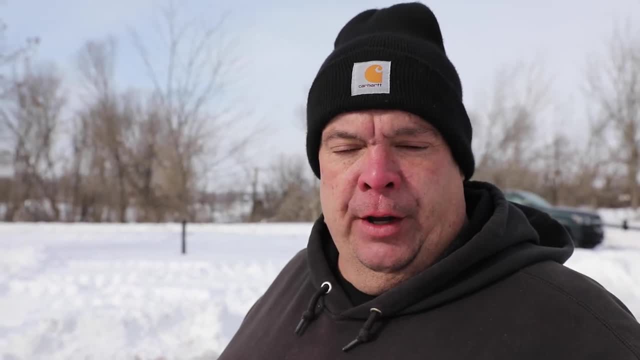 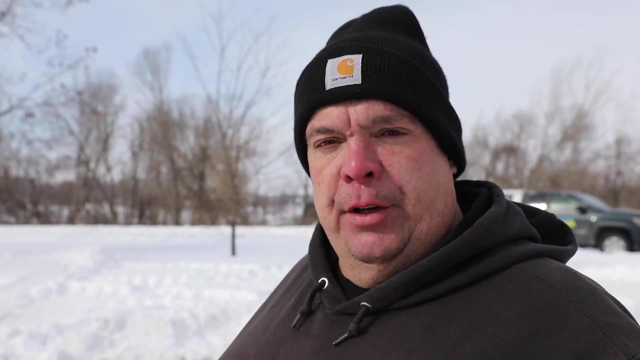 they're bigger or exposed, And then you have rot or faster-grown trees which have a heavier soil. So you know that's where the pith will be in all kinds of different boards which affects sapwood, which is kind of a common defect, depending on where the tree's growing more upland. 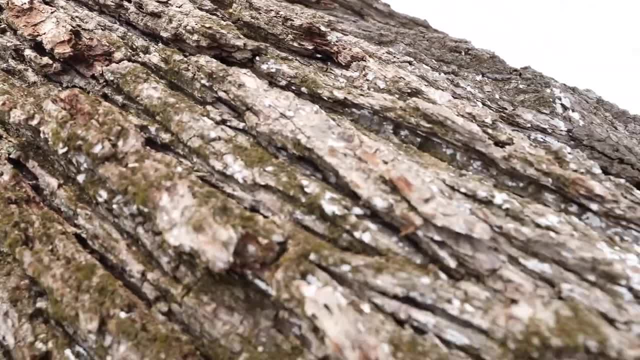 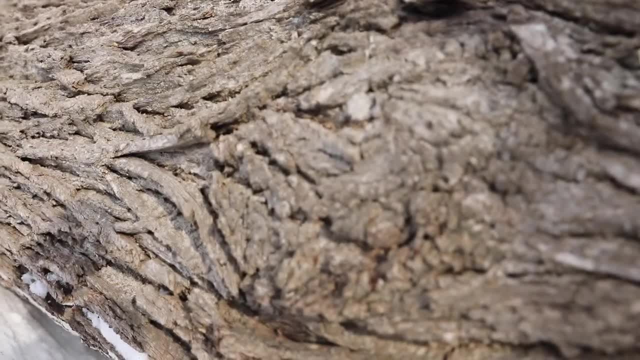 or in the bottom I mentioned. you know what a catface was and here, if you look at this log right here, you can see it's a big, it's a wound that was covered up by a, you know, a limb, And 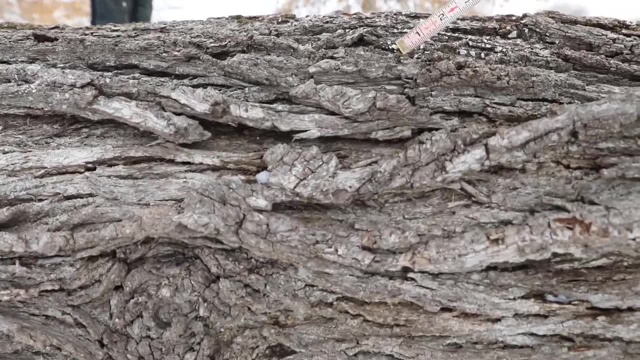 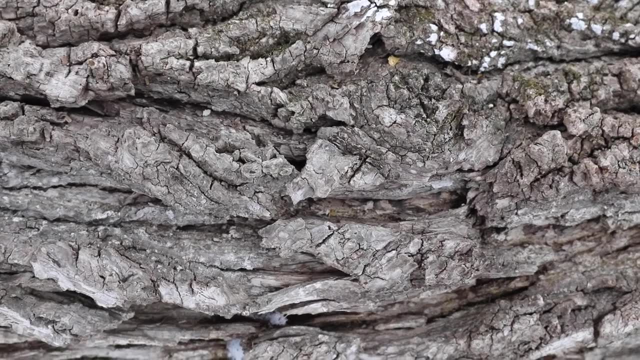 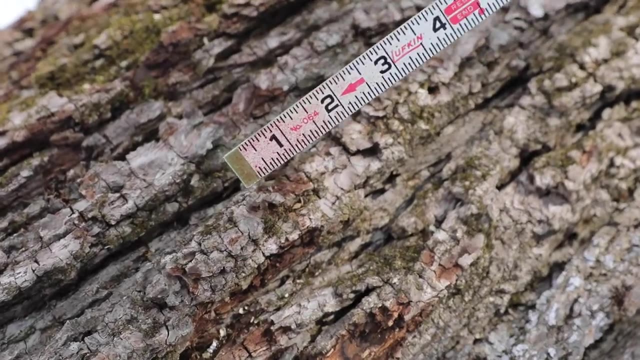 then here's more of what you'd call a pin knot. You can barely see it, but it's usually circular in the bark And then up here is a cross And it usually grows in the end of a, in the top of the tree, And it a lot of high-end furniture. 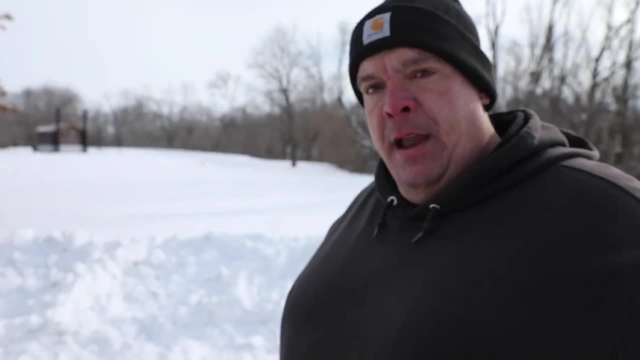 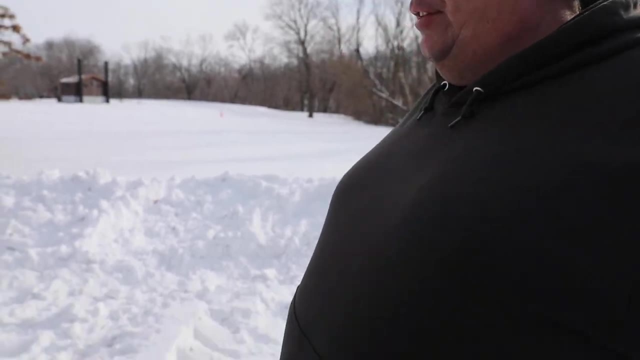 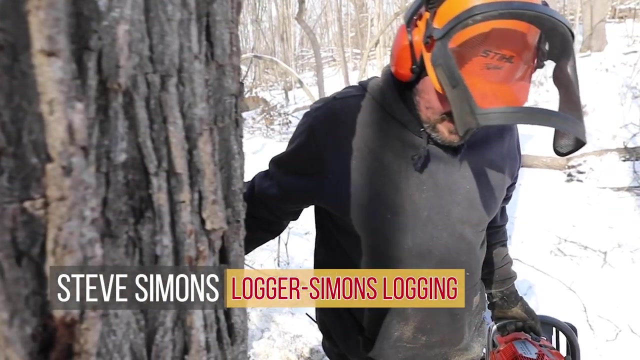 you know, instruments and such get made from this material. It kind of looks like a rattlesnake back and it kind of goes through the saddle up here And usually they try to keep it on a bigger log and it's usually it's pretty cool to see Proper timber. marketing involves foresters, loggers. 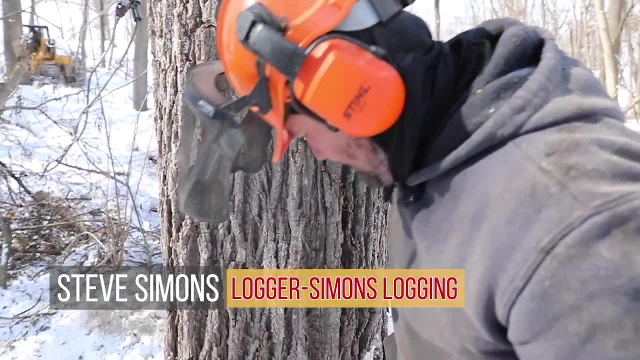 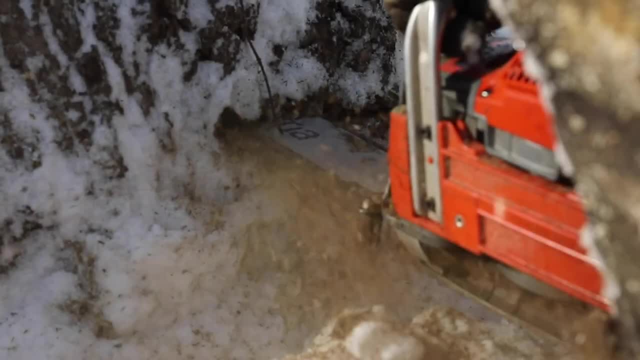 and timber buyers, And that's what we're trying to do here. We're trying to make sure that we're doing that. for foresters, Knowing the roles and skill sets of these equally important yet very different occupations is critical. Well, Ben, there's a lot of players that go into timber. 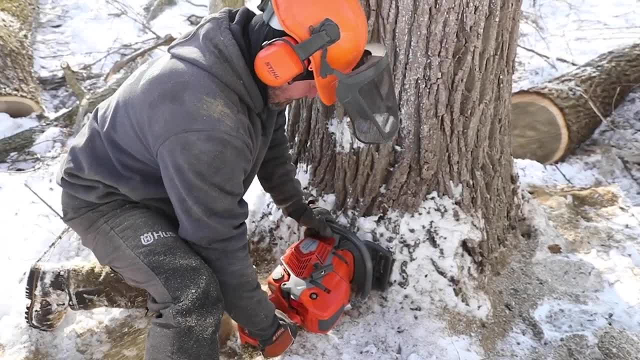 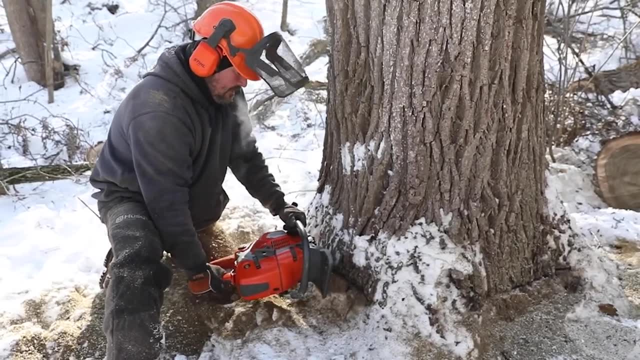 sales and timber harvest. There's foresters, there's loggers and there's log buyers, So most folks don't know the difference between those. Could you explain those? A forester is usually somebody with a education or degree in forestry, and typically foresters. 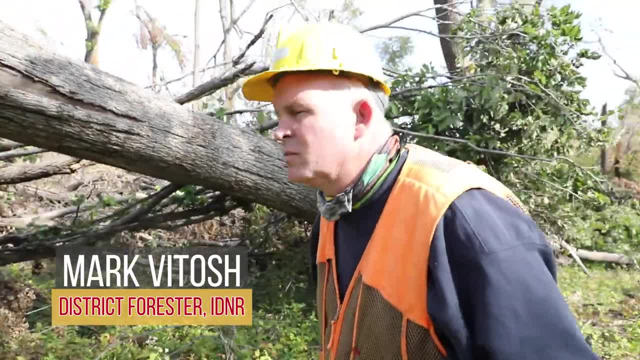 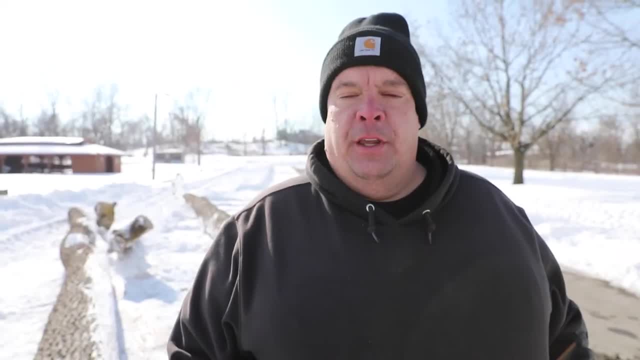 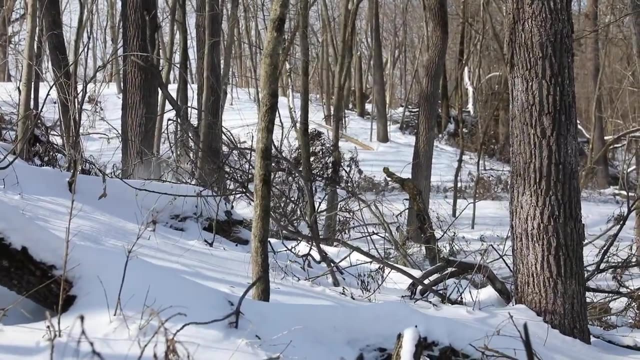 are looking out for the best interest of the foresters And they're looking out for the best interest of the landowner or the longevity of the land. you know the good steward Loggers are, you know they cut the trees and you know, get the trees to the landing And a log buyer or